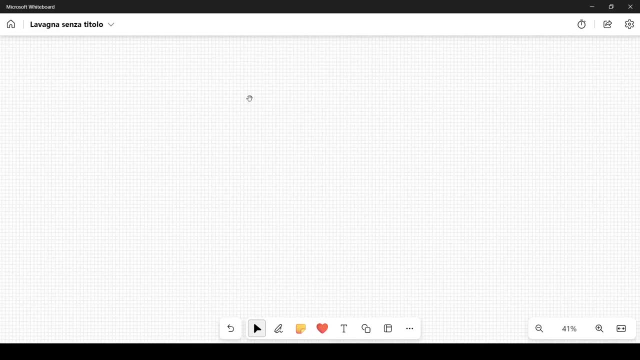 A spin 1 half particle is associated with the Dirac Lagrangian. In this case, let me write the Lagrangian like this: So we have LD, which stands for Dirac. so L stands for Lagrangian, D stands for Dirac. 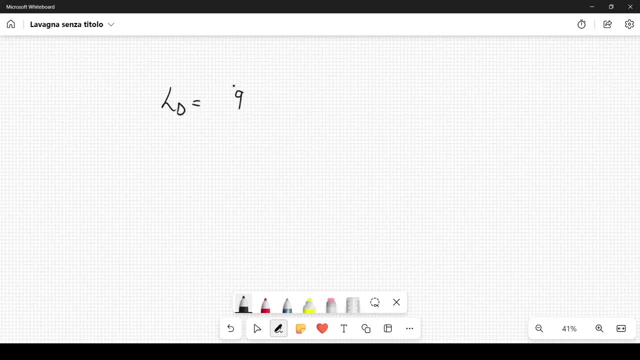 so we have the Dirac Lagrangian. Here we have the following field: QF bar. so I will call it like this and I will tell you why. And then here of course, we have I gamma, mu del mu. so you can also write it like this: 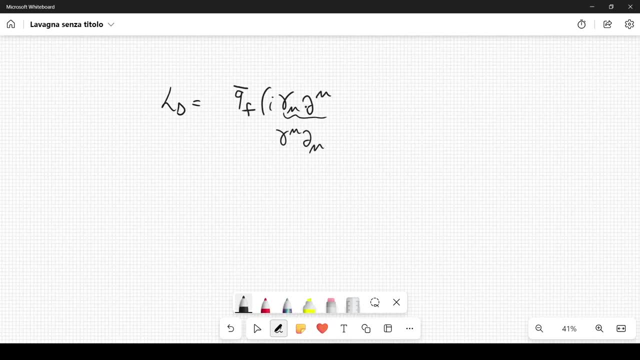 if you want gamma, mu, del mu- Raising lower indices is something that at this point you should be comfortable with- You have to use the metric tensor. Then we have minus MF, so this is the mass associated to this field, And then we have QF. so, in general, when we have a certain theory, we have some fields. 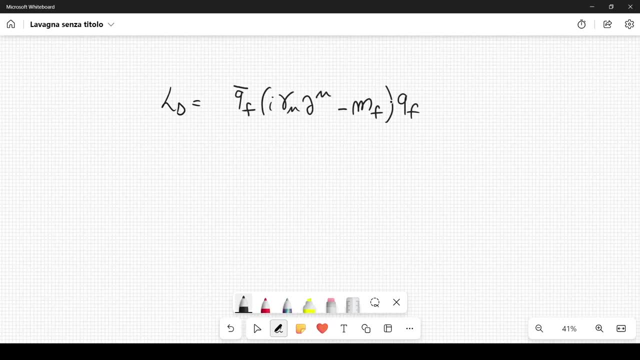 the excitation of these fields will be particles, and these particles have some mass, and in particular for the Dirac particle we have the mass MF. Then we have to sum over F here. so we are going to sum over F, and let me tell you what. 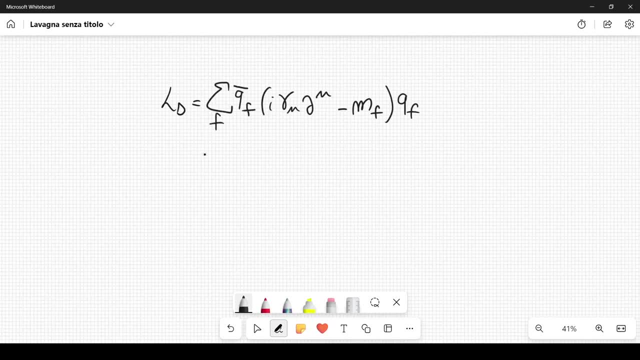 F stands for. F stands for the flavor, The so-called flavor. It's another property of particles. There are different quarks filled with different masses and therefore different flavors. In particular, the different types of flavors that we can have are the following: 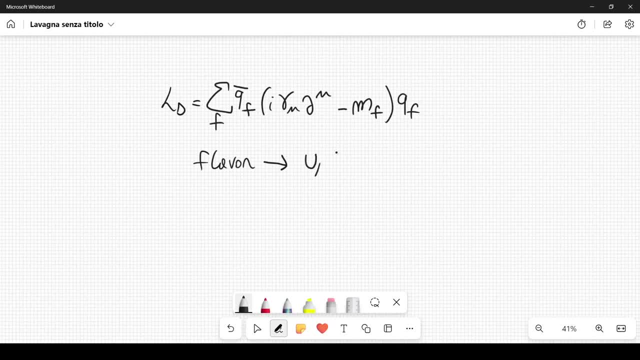 We can have the up quark indicated with a U, then we can have the down quark, then we can have the top quark, the charm quark, the strange quark and the bottom quark. So we have six different types of quarks. 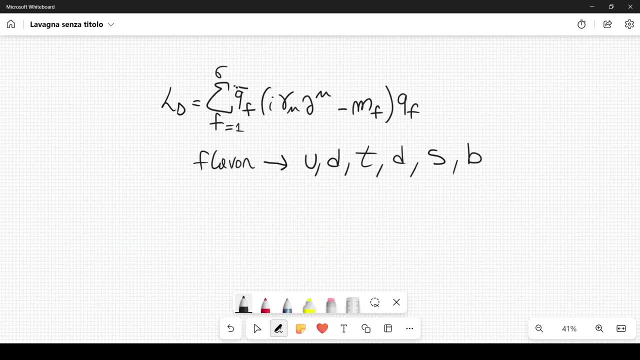 We have different types of flavors, so this summation can go from one to six. This is how you can think of these flavors. These different flavors arise from years of experimental and theoretical evidence. Then let me tell you something more about this QF. 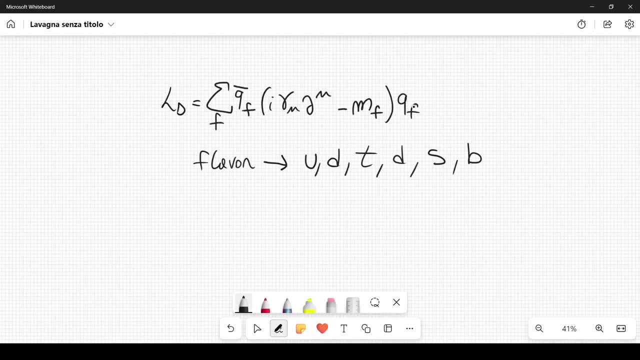 So Q stands for quark, F stands for flavor and, in general, for each quark we can have different masses for the different flavors. Okay, Okay, Okay. So QF can be represented in different spaces, In particular if we consider the spinorial representation of QF, since we know that its 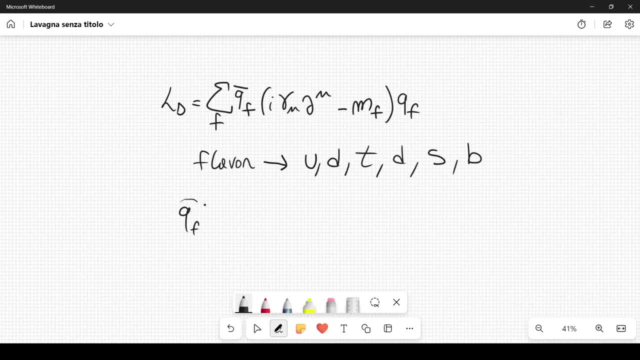 spin should be equal to one half. this can be also represented as a spinner When we want to emphasize the spin of the quark, because we can act with these matrices, on these states, on this particular object. let's call them that. 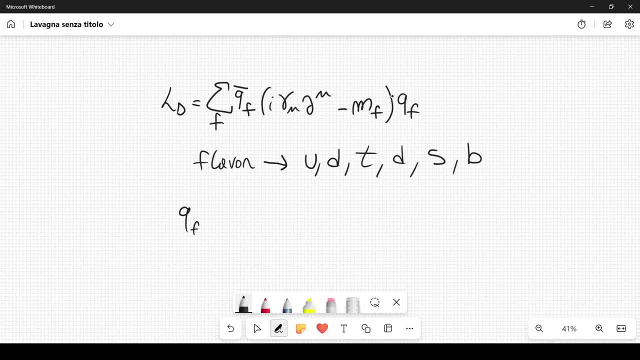 Okay, So we can represent them with the four components that usually one associates with this type of object, But at the same time we can also represent these quarks with the following three components: So we have QF1,, QF2, and QF3., 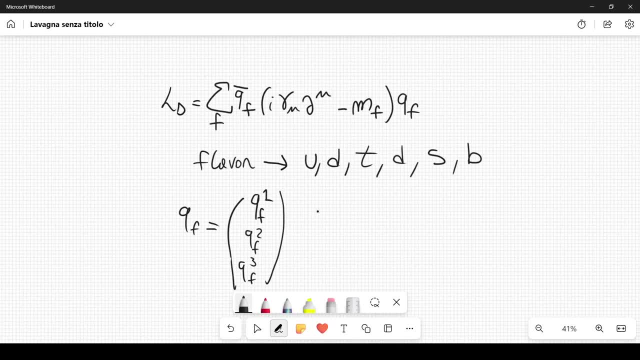 So this is a different representation and, in particular, this is also called the color representation. Okay, Okay, So let's look at the quark. Okay, So what is the color representation? Because each quark can have three different colors and this is associated with the SU3,. 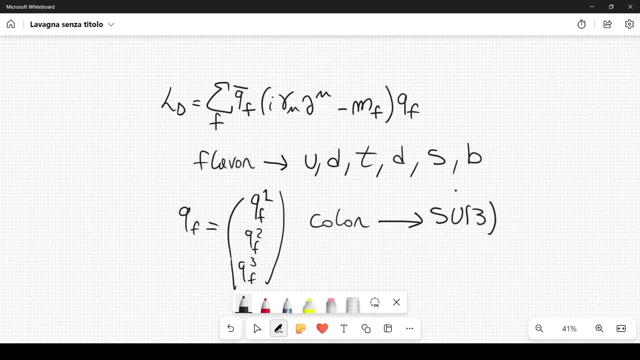 the special unitary group in three dimensions. You have to think that the so-called color, which it doesn't have anything to do with an actual color that you can see with your eyes, but it is just a term. so this color used to make an analogy with the concept of charge for the electron you can have. 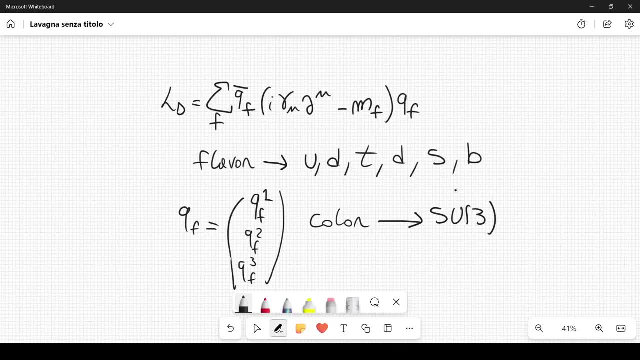 either the charge of the electron, but I remember that in general, when you consider the Dirac Lagrangian, you also have the anti electron, which is the positron, and therefore you have to consider the, the opposite charge in this case. we are in su3, so we can have different three types of colors, so you 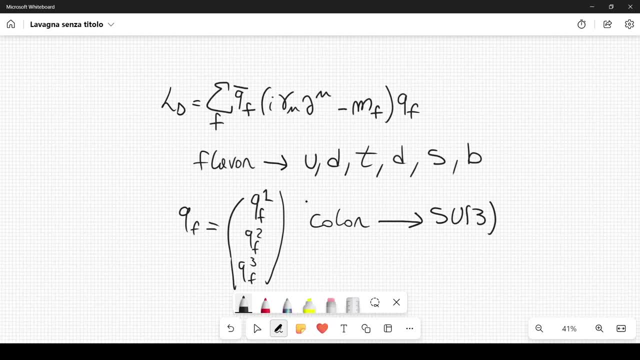 can think of them as three different types of charges for the for each quark when we consider the color representation. so when we are making our considerations and which are related to the color of the quark, we have to use the su3 representation so the quark transforms according to su3. so we need 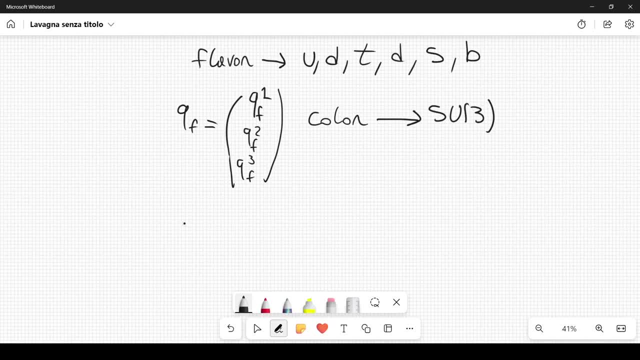 to use special unitary matrices in three dimensions. in particular, we can write Q alpha prime F equal to U alpha beta, Q beta F. so we apply a unitary matrix to this field. so we can use the- in this case I'm using beta- to denote the color index. 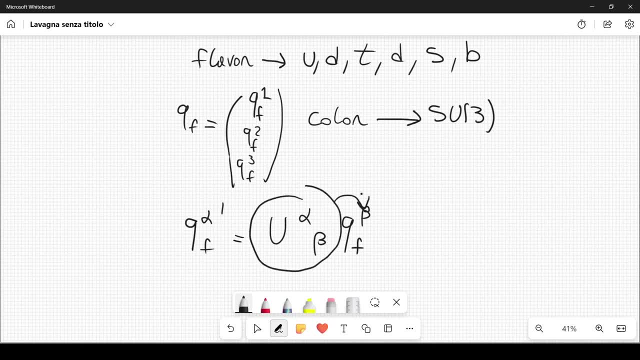 therefore, this matrix will only act on the color and you will get. you will get another field which has a different color in general, so you are applying this transformation to is a state, or let's call it a quark, and then you can have a transformation of this kind where the color changes. 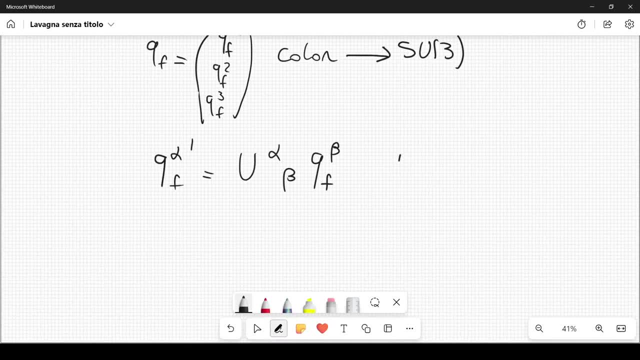 the matrix U is unitary, so it means that U U dagger is equal to U dagger, U, which is equal to the identity, and you can be written in the following form: so we have e to the minus, I GS. GS is just a constant. then we have lambda a over 2, theta a, where a is an. 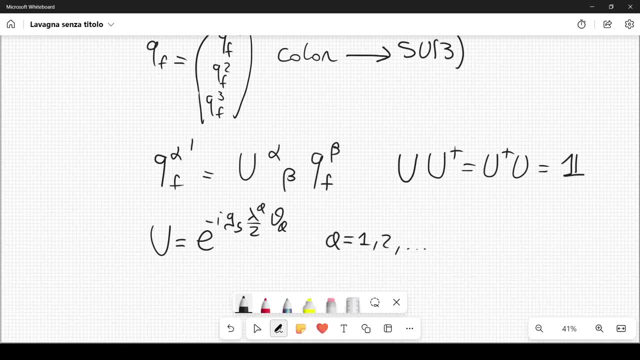 index that ranges from 1 to 8, because remember that we have the special unitary group in three dimensions. therefore, there are eight generators and the lambda a's are matrices, so lambda a denotes the generator, the eighth generator of the fundamental representation of the SU 3 algebra, the 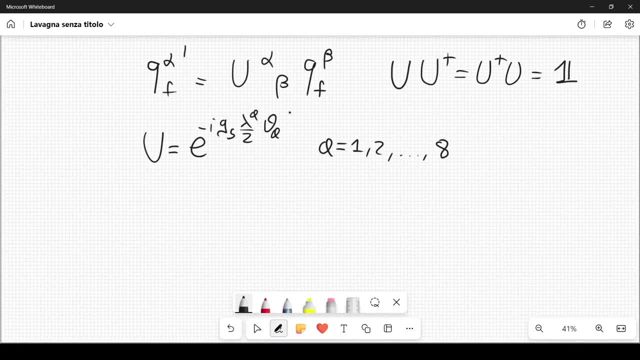 matrices lambda a are traceless. these matrices here are traceless and they satisfy the following commutation relations. so we have lambda a, lambda B, commutator equal to 2i. so this is the imaginary unit. then we have F ABC, lambda C, and this F ABC are the so-called structure constants and they are real and totally. 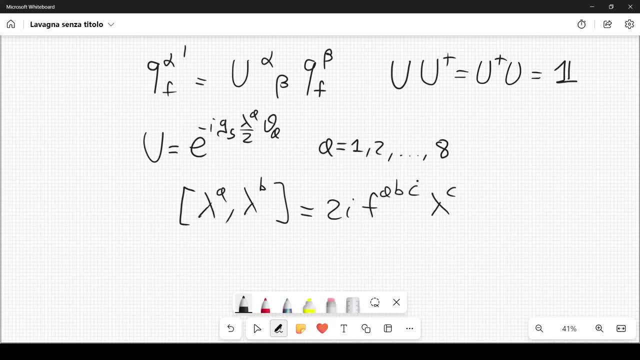 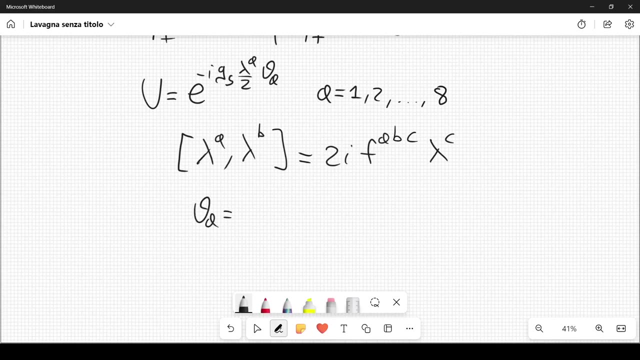 anti-symmetric, as we have seen, as in the QED. so quantum electrodynamics case, we can require that the Lagrangian be invariant under a local transformation, that is, when theta a these parameters. here they depend on the space-time coordinates. so this is a very important parameter and we can use it for the 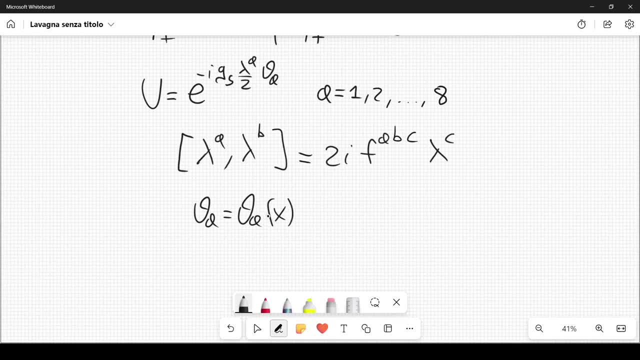 function of x, theta a of X, and to satisfy these requirements, so to satisfy the fact that the Lagrangian being variant under a local transformation, we need to change the derivatives to covariant derivatives. and since we have eight independent parameters- theta a, we need eight different fields and we will 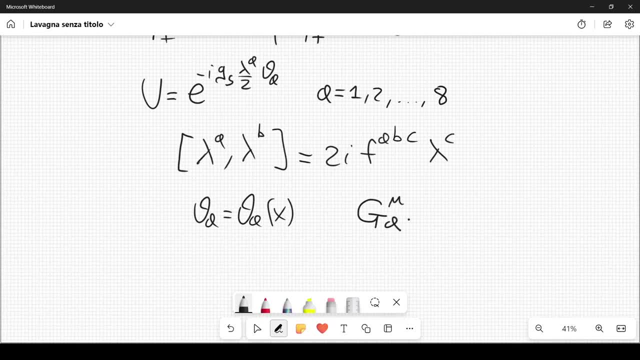 call these fields G, mu, a of X. so when we change the index a from 1 to 8, we have 8 different fields. remember that we also need this index mu and I will remind you why we also need this index mu. it's very simple to motivate that. 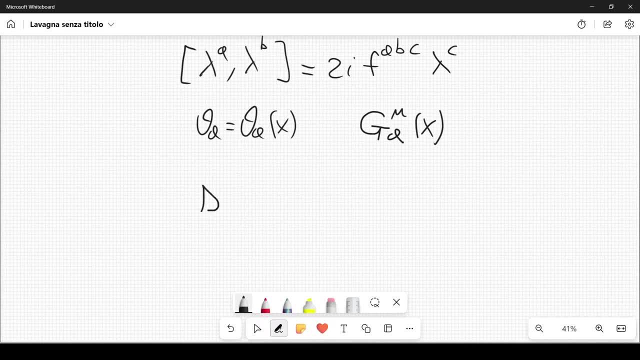 because we define the covariant derivative d mu, applied to QF, like this: so we have d mu, so this is the usual partial derivative minus i gs, lambda, a over 2 g, mu, a, x, and we apply this, of course, to QF, so you can think of this as a definition. 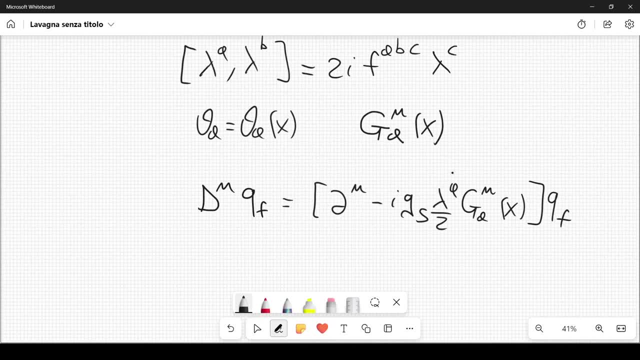 but this is reminiscent of what we did in QED, and let me also tell you that these fields, these 8 fields, are called the gluons, which is important in quantum chromodynamics. that is the theory that we want to describe here in this lecture and in the following. 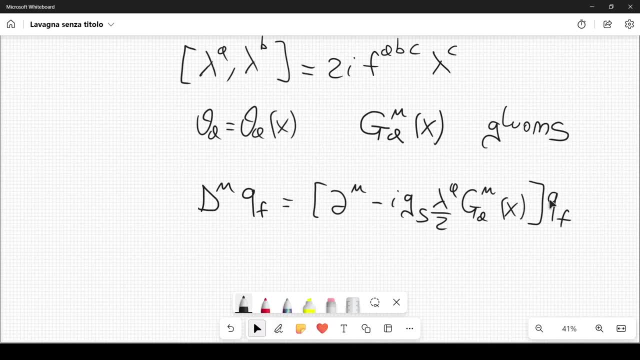 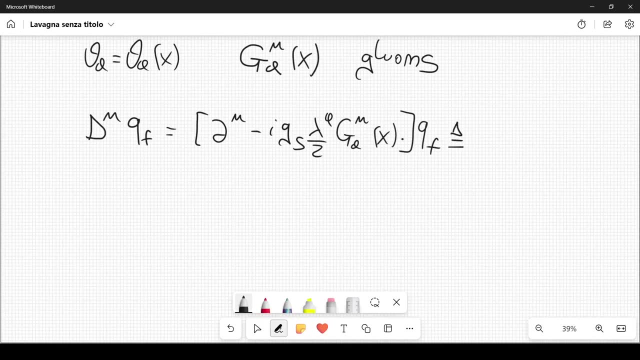 it's a part of the standard model, so it's very important for us to understand it. so we can also define this in the following way: in particular, we can put together these matrices lambda a with these scalars, so we have to think of these as scalars. 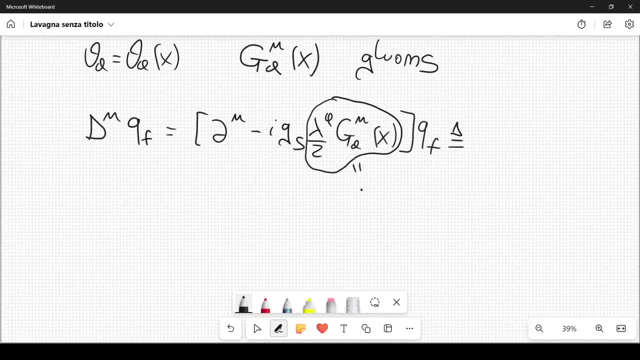 these gluons. we can define them to be g mu, so this will be g mu of x and it will depend on the two indices of this matrix. so there are some hidden indices inside this matrix, because remember that this is a matrix, so each lambda a is a matrix. 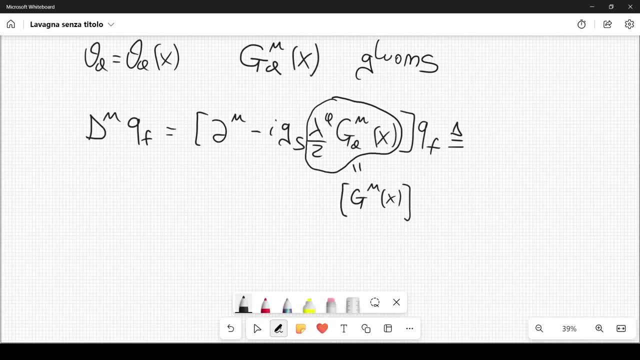 so there are also two hidden indices that we can call, for example, alpha and beta, and here there are two indices, alpha and beta as well, so we can also write this as lambda a over 2. and then here we have two indices, alpha and beta, and then we have g, mu, a of x. 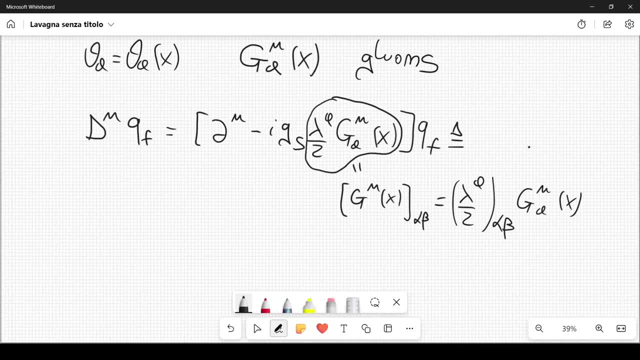 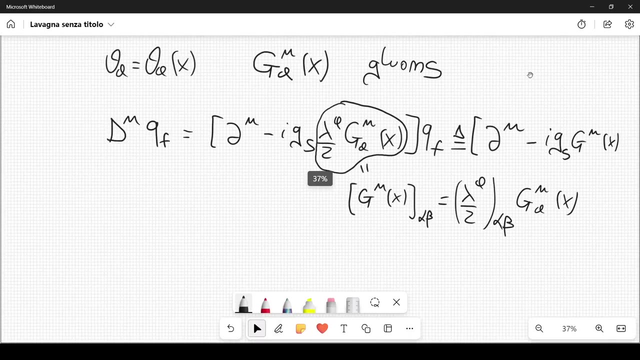 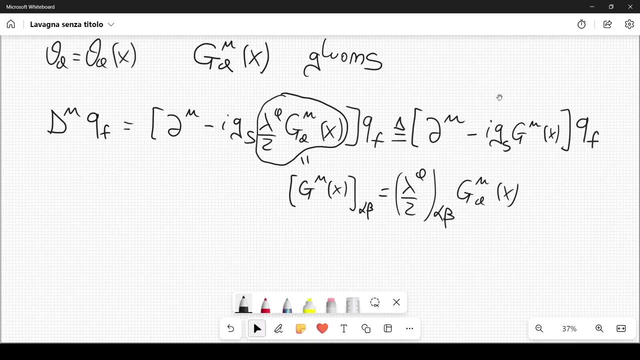 so remember that in this case we are summing over a and therefore we can define this covariant derivative also like this: g mu minus i g s, and then we have g mu of x and of course then you have a qf here. now we want: 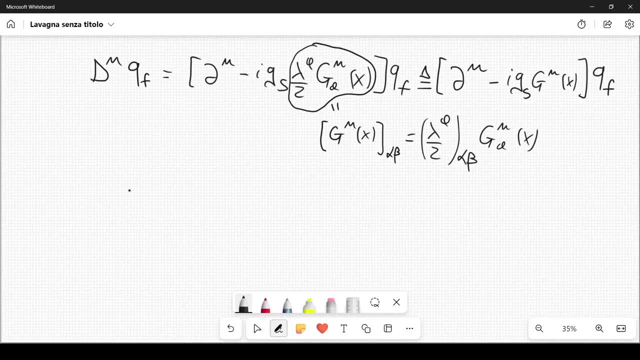 so we want to define the covariant derivative in such a way that it transforms in the following way: so g, mu, qf. when we transform it, so when we transform this- and i will put this prime to indicate that we are going to apply a transformation- this should transform in the following way: 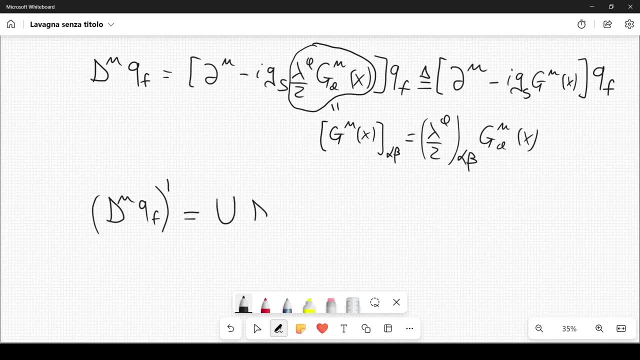 so we have the unitary matrix u, and then we have d, mu, qf. so this is something that we are going to impose. we will see why, but it is something that you can understand also from what we did in qed, in the qed theory. so if we impose this condition, 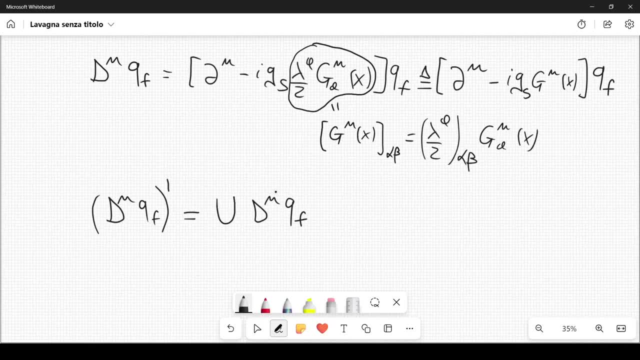 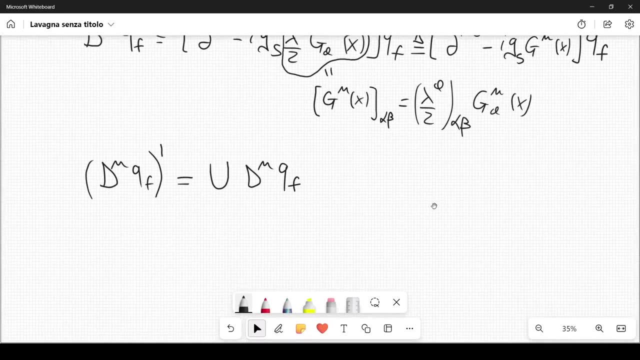 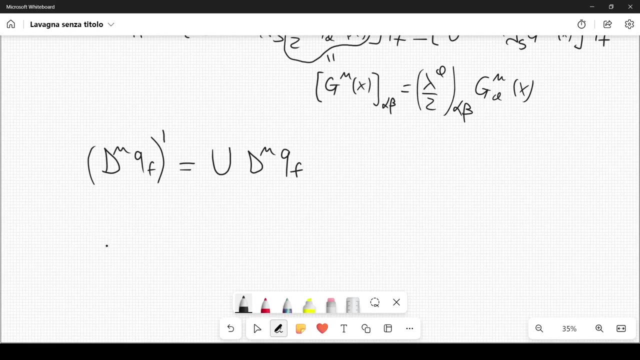 this will, in its turn, impose a transformation on g mu, and we are going to see why. so, so, so, so so. in particular, we have the following: so d mu, qf prime, this is equal to del mu minus i, g s, g mu, and in this case, this has to transform. 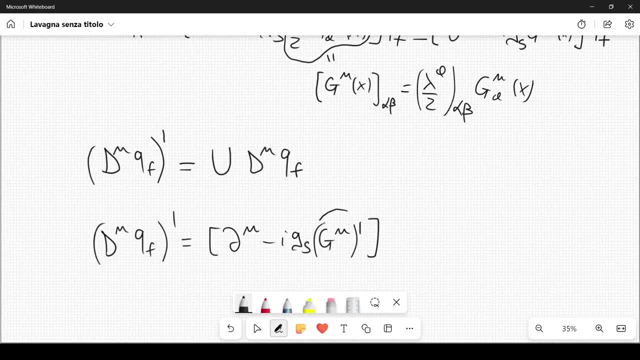 because it's the only thing that's going to transform. it's our field that's going to transform, just like in qed, we had a mu, so and then here we have the transformation of qf. so we have qf prime, but qf prime can also be written as u, qf. 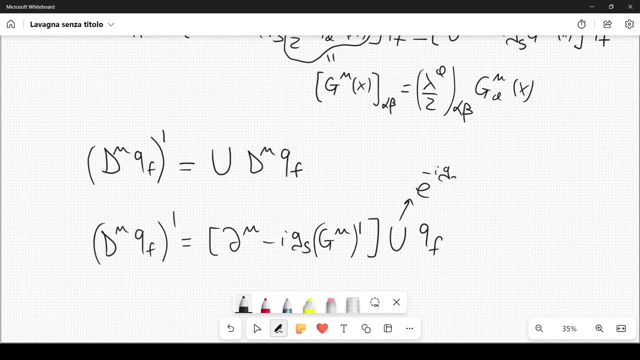 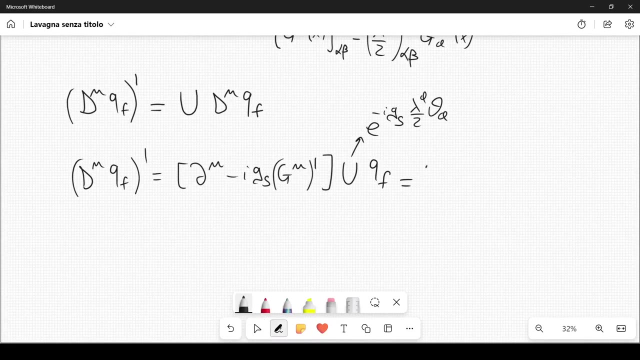 and remember that u is equal to e to the minus i gs. then we have lambda a over 2 theta a, so we want to impose that this is equal to u. and then we have lambda a over 2 theta a, so we want to impose that this is equal to u- qf. 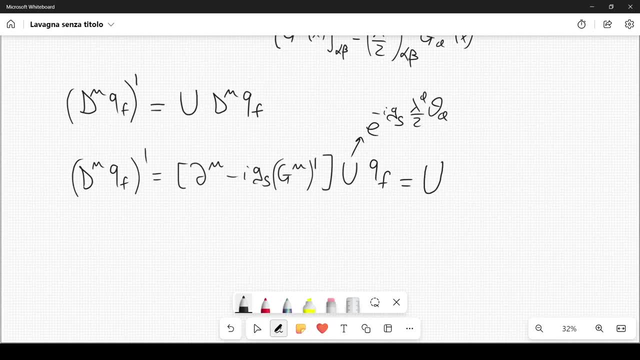 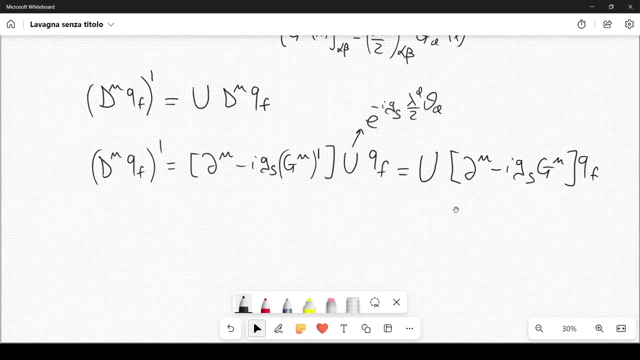 and then we have this right, so we have d mu, which is del mu minus i, gs, g mu, qf. so i know that this kind of notation can be not so easy to follow all the time, despite, i mean, we have gone through the reasons why we should do something like this. 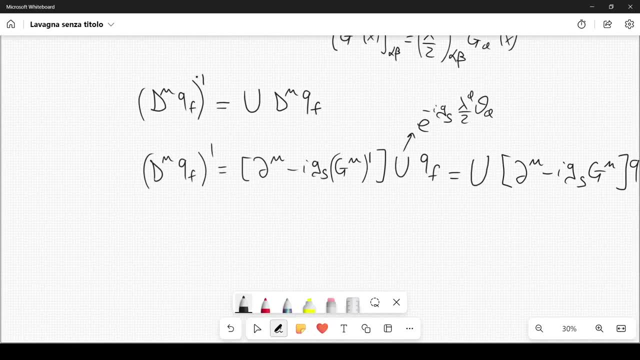 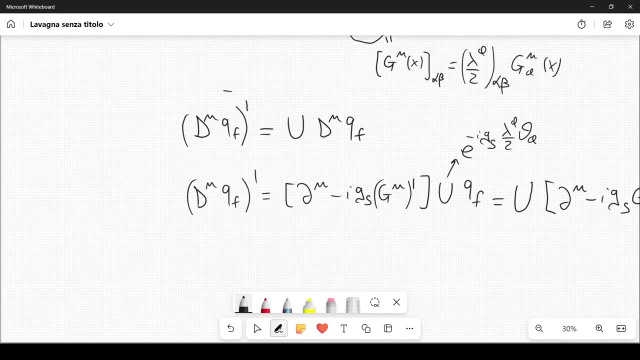 let me tell you once more why we should do something like this. i mean, why do we have to impose this condition here, here? it's not complicated to understand that, because remember, remember that in our theory, if we impose something like this, just like mean qed, remember that. 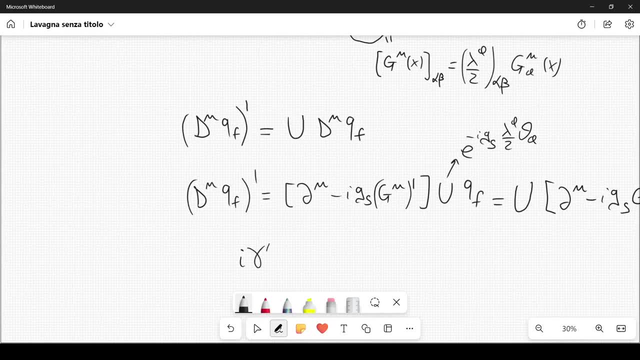 we have terms like this- we have i, gamma, mu- then here we have to replace the partial derivative with the covariant derivative. so in this case i'm going to write mu as a lower index here. but don't get confused by the position of these indices. you just have to think that you have. 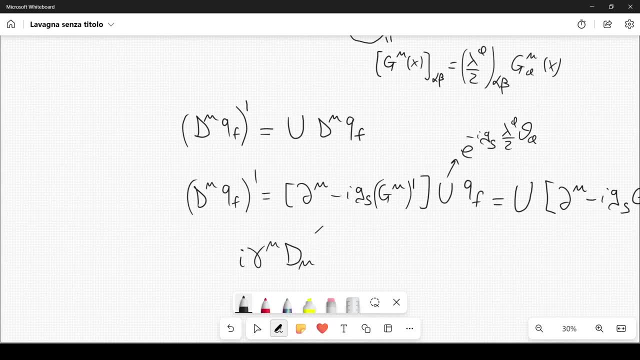 you can apply the metric tensor and you can reasonably understand or make sense of these positions here. that's not a problem. remember that we have something like this: so minus mf. and then here we have qf, and here we have q bar f and you're going to sum over f, but that's not the point. so if we consider the second part, 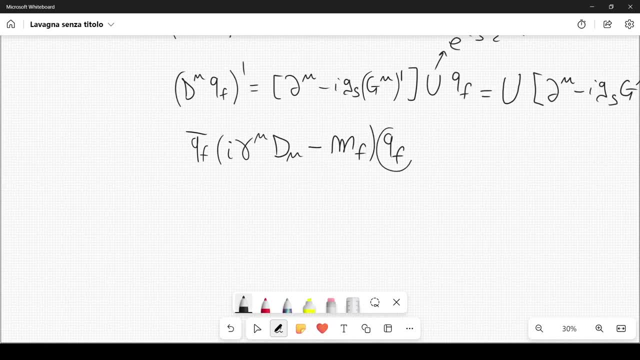 so when we multiply qf bar by mf and then qf, you have something like qf bar qf. so when you impose the transformation of the kind qf goes to qf prime, i mean qf becomes qf prime and this is just u applied to q to qf. so when you consider q bar, 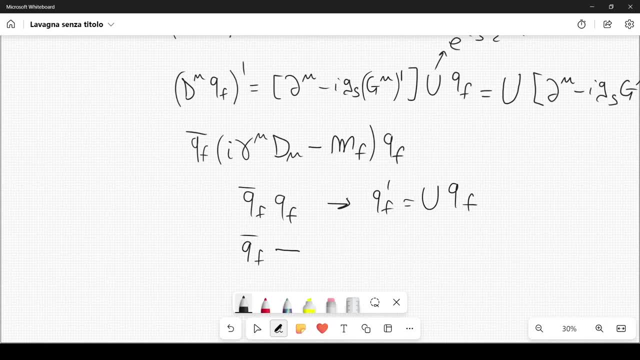 when you consider qf bar, this will transform like this: it will become q bar f prime and this is equal to qf bar u dagger. it's simple because you can understand it from here right. i mean, if you take the dagger of this, you get qf prime dagger. then you get qf dagger u dagger. 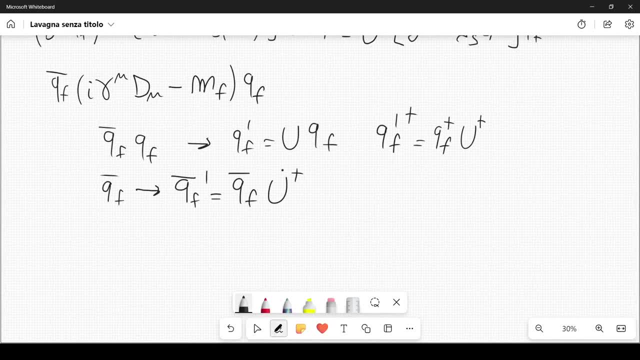 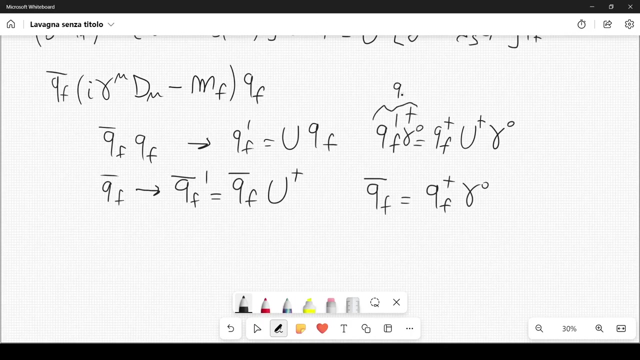 but now, now, at this point, you have to remember that q bar f, this is just qf dagger, gamma zero, right? so if you act with gamma 0 on the right here and also on the right here, this part is just qf bar prime. and also notice the fact that gamma 0 here, which is a dirac matrix, can commute with this operator. 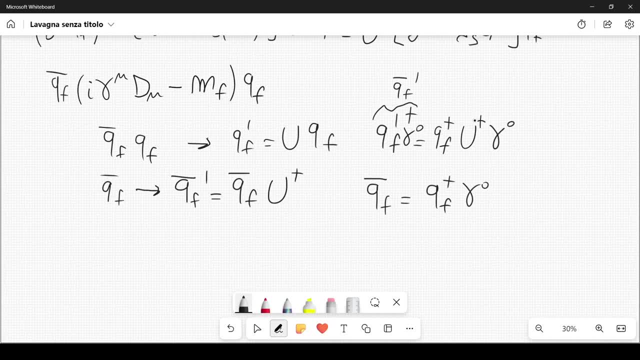 u dagger, because u dagger is something that acts on the color. remember that we have the matrices lambda a, lambda a, which are three by three matrices, so this operator u dagger, so they are three by three matrices in that kind of representation. remember that that we are using 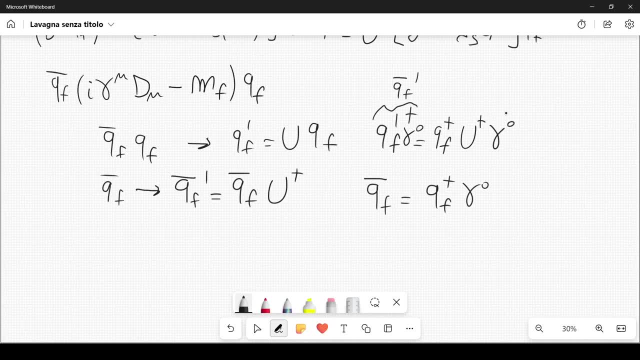 representation or different representations. the gamma gamma matrices usually are represented in a four-dimensional space, but these matrices act in a different space with respect to these ones. so we can also put this gamma 0 here on the left of u dagger, so this can also be written as q f. 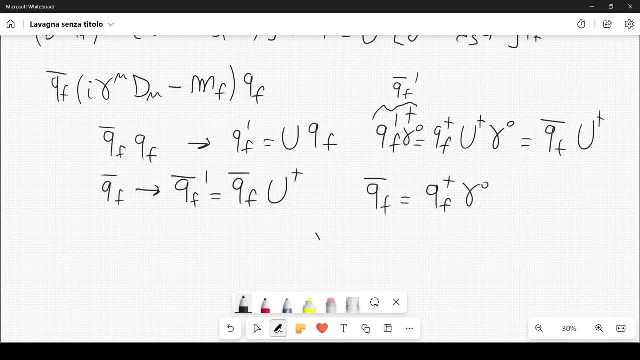 bar u dagger, right. so that's why we have this kind of transformation and therefore, when you consider qf, q bar, f prime, q f prime, this will be exactly equal to q bar f, q f, because you have u dagger u, which is, of course, equal to the identity. 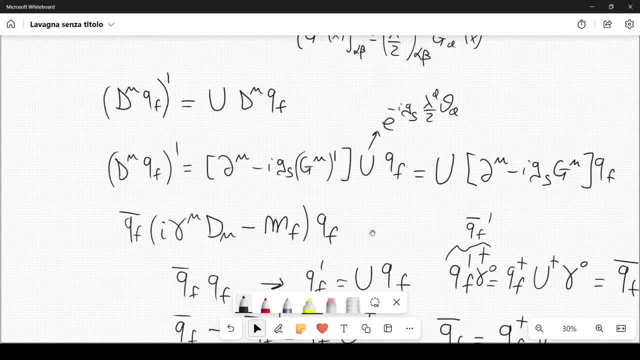 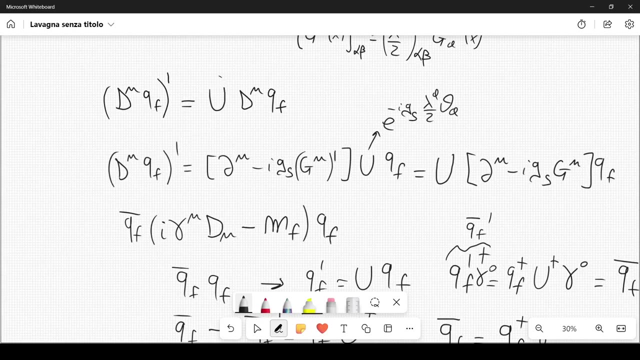 and if we impose this transformation here upon the- this is a coherent derivative applied to qf- then we- i mean we- can make sure that our lagrangian will remain invariant with respect to this type of unitary transformations. so that's why we want such transformations, because 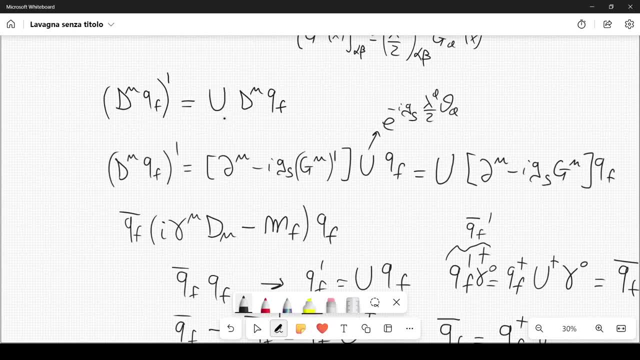 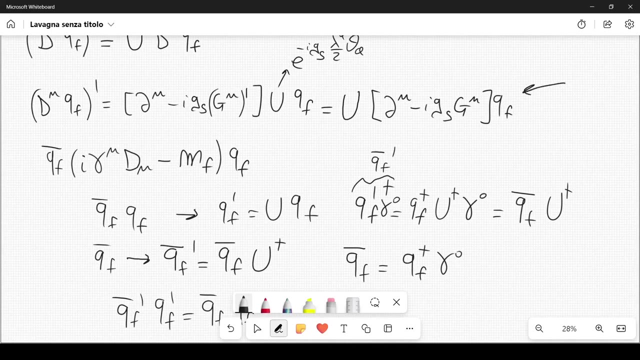 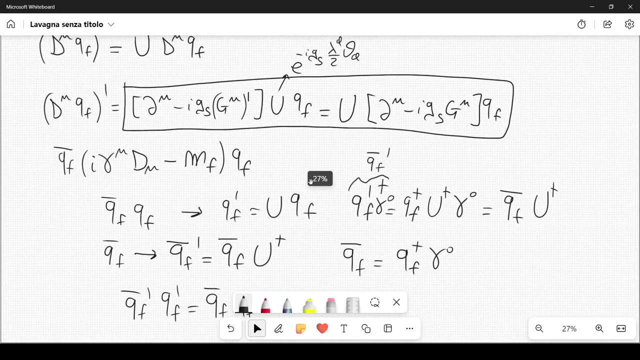 the lagrangian will remain invariant, and it is something that we have already done also in qed, with different types of transformations in that case, but that's the reason why we're doing that. so we impose this equality and from this equation here, from exactly this equation, we can find the transformation of for g mu prime. 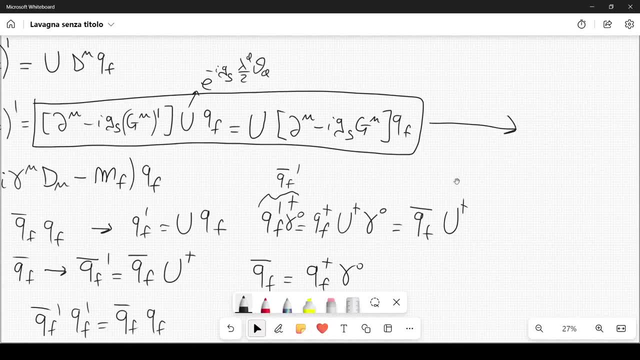 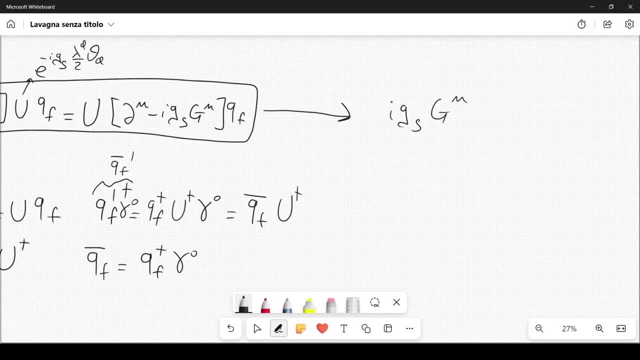 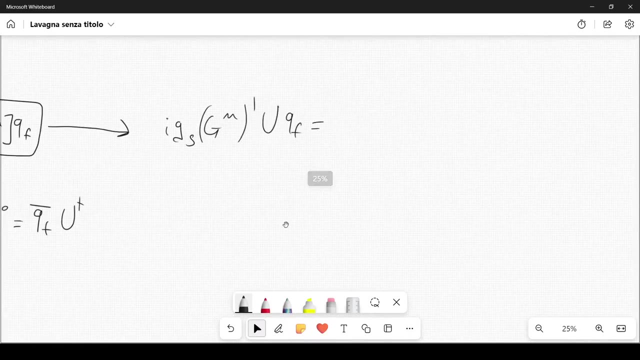 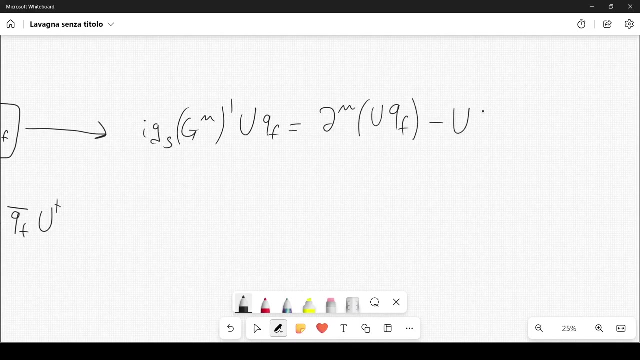 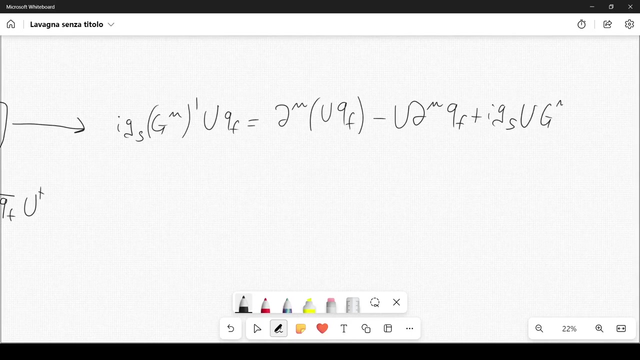 so let me rewrite this so we can write i g s, g, mu, prime u qf. and this is equal to to what? to dµuqf minus u delµqf, and then we have plus i gs, and then we have u gµqf. 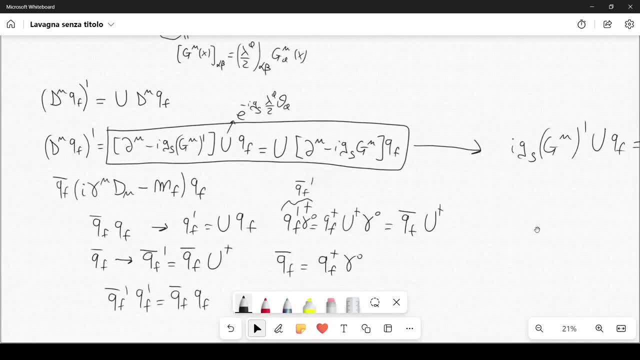 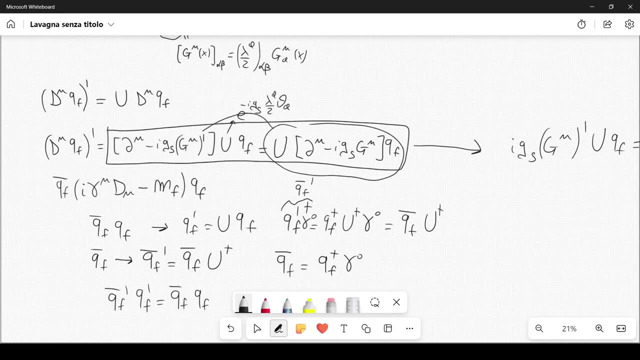 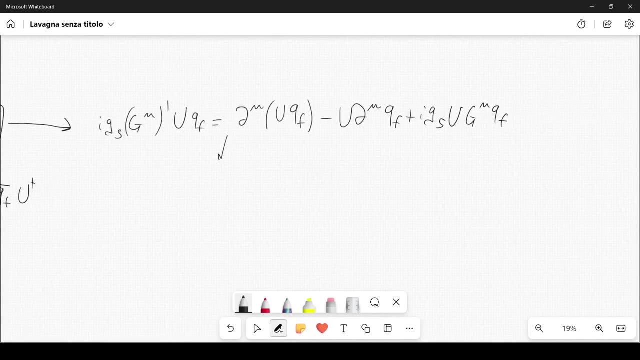 so i have simply isolated this term, so i have put this on the right and then i have put these terms on the left, and this is something that you can write from here. now you can see that these two terms can simplify a little bit, because they will give you dµu and then you have qf. 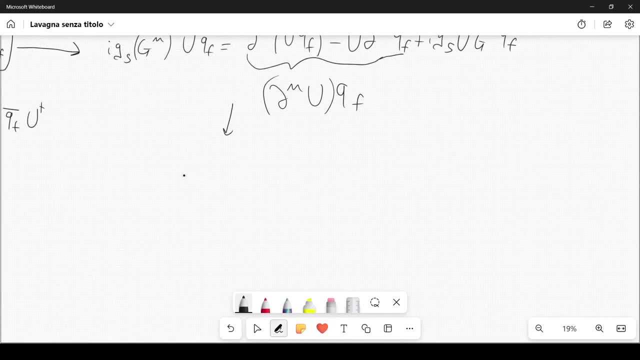 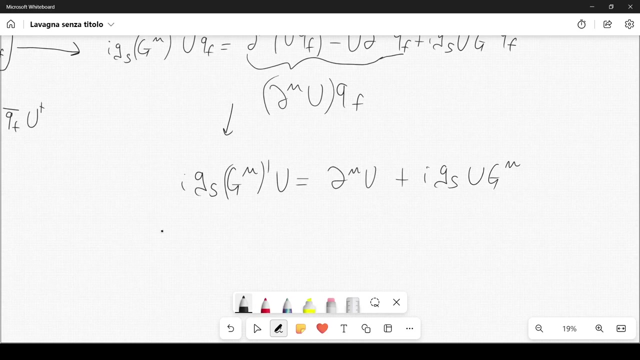 so, all in all, what you get is this: what you get is the following equation: you get i gs gµ' u equal to delµu, plus i gs u gµ, like this, and therefore you get the following: so you get the following transformation: gµ'. 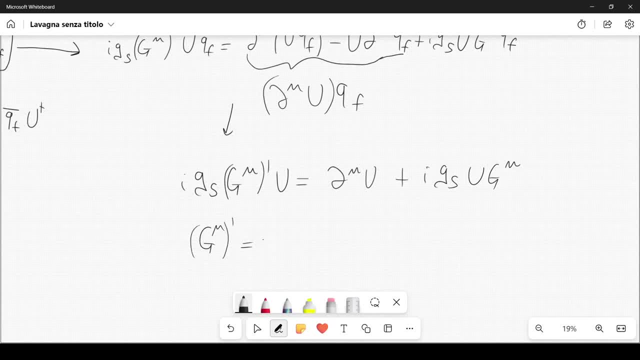 gµ' equal to minus. i dµu u dagger. we divide by gs plus u gµ u dagger. so it's quite simple to get from this one to this one. you divide by i gs and you also have to act with the? u dagger on on the right. 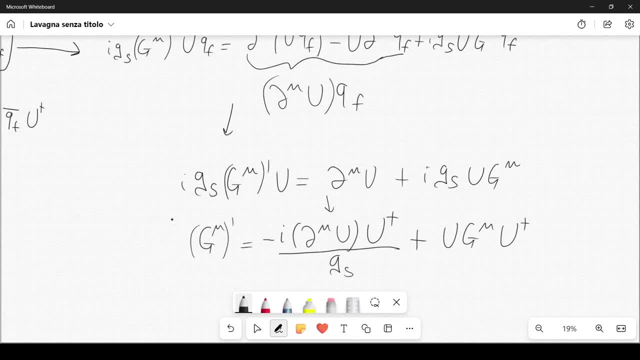 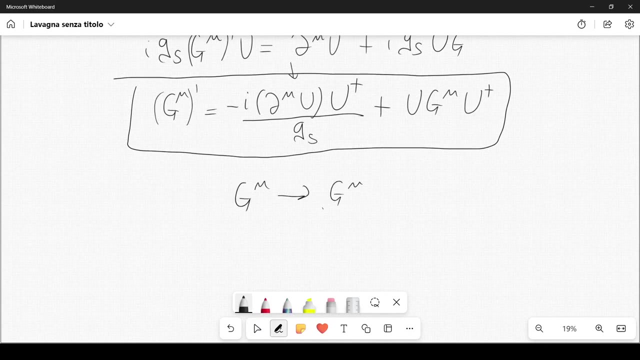 so this is what you get and this is basically the transformation that we have to impose gµ' on gµ'. so gµ' should transform just like this: i have gµ which goes to gµ' like this, and the transformation is that then we have qf which goes to qf'. 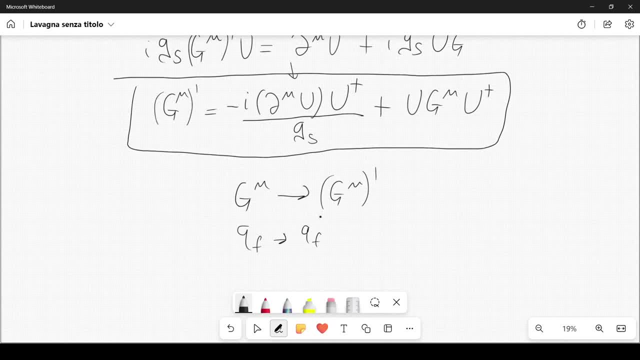 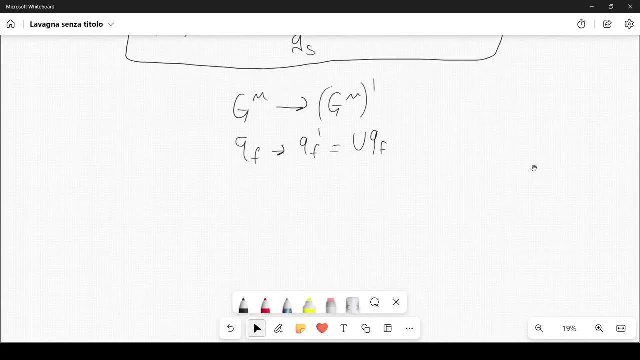 then we have qf, which goes to qf', which is equal to uqf, and then we also have the covariant derivative gµ', which goes to qf', y, qf', so this is the indeterminate term- and then we have 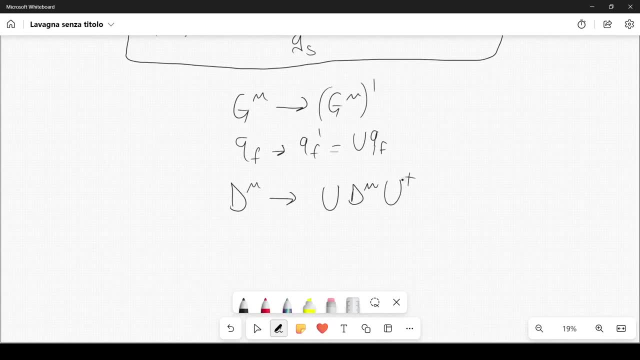 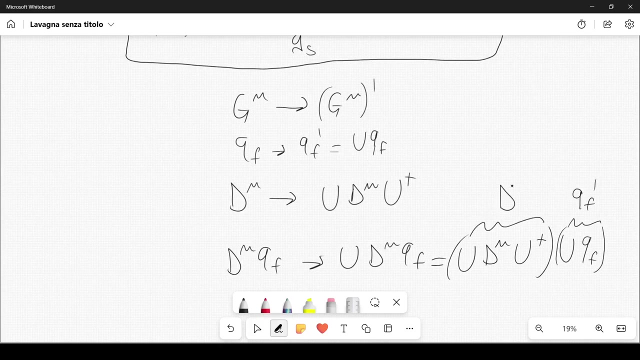 which goes to u d mu u dagger. why is that? why, I mean, why do we have to impose this? well, it's quite simple, because d mu QF transforms as u d mu QF, and since QF transforms like this, this is equal to u d mu u dagger, u QF, and this is just QF prime, and this is just d mu prime. so, 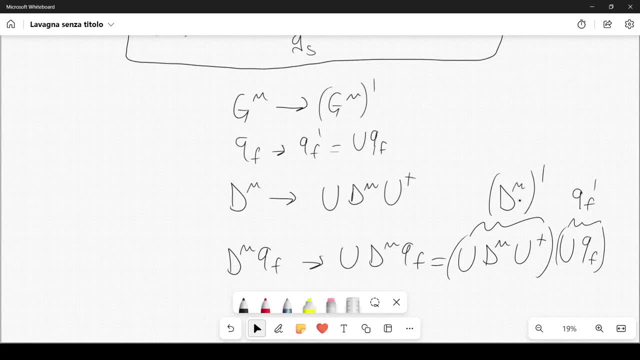 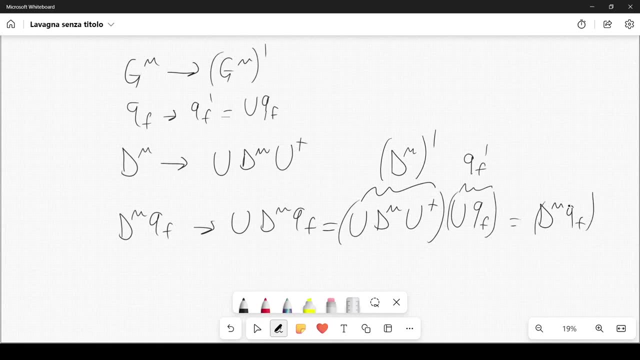 this is the transformational. I mean, this transformation here is exactly the mu QF prime, like this. so these are the transformations that we have and we will proceed further next time, because I don't want all, the all these lectures to be too long and it's necessary for you to be.